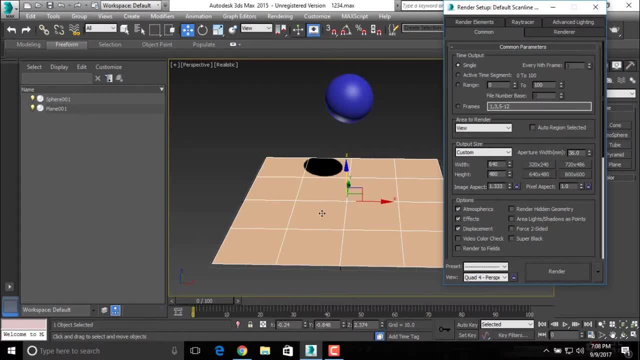 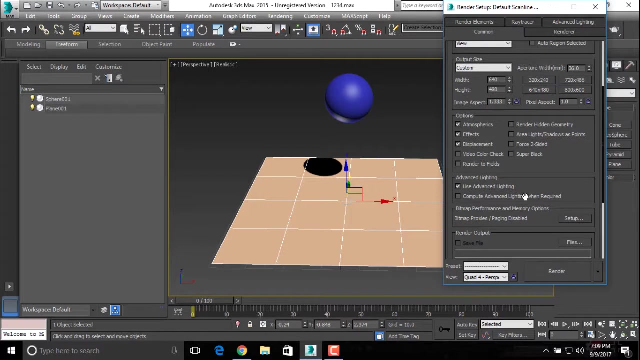 many option. now we want a animation from 0 to 100 frames, so click on the active the time segment. in the active time segment we can get the animations for a 0 to 100 frames, so our frames are run 1 by 100 times, 0 to 100 times. and now we want output as a avi file, so click on the render. 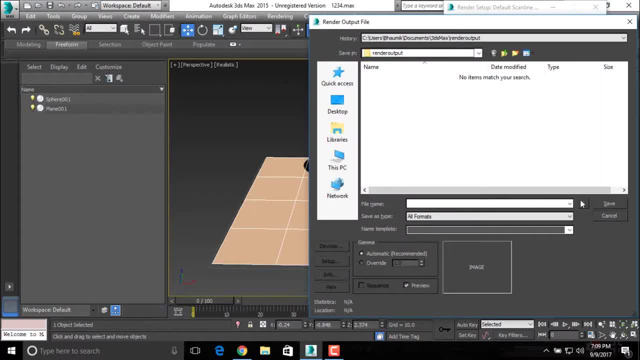 to the output files and select your path where you want your output. so go to the any path where you want your output to be. so go to the any path where you want your output to be. so go to the any path where you want your output to be. so go to the any path where you want your output. i am saving at. 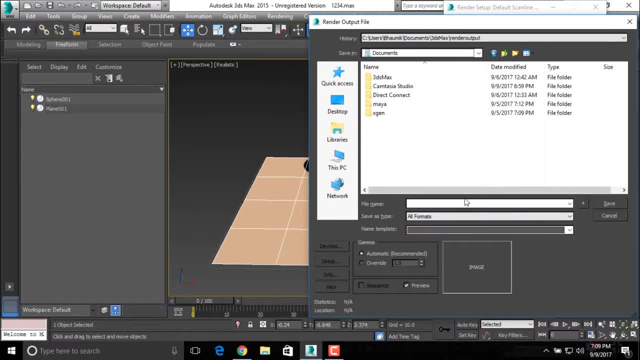 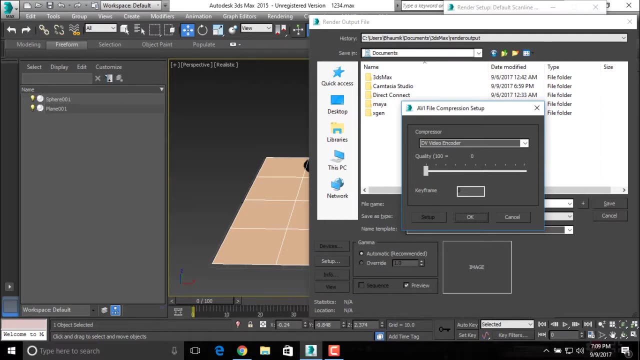 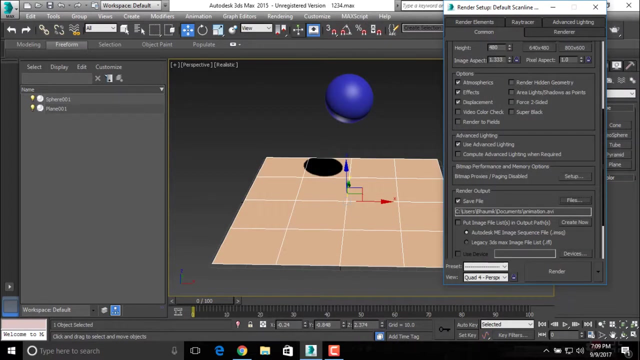 want your output. i am saving at the document, so here i am output as a animation and select the output format. i am selecting the avi format and press save. after click on the save, it's give you the settings. what type of settings you want to do. just click on the ok. now, if i am click on the. 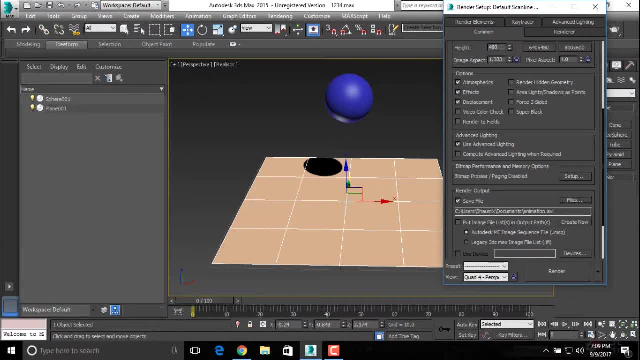 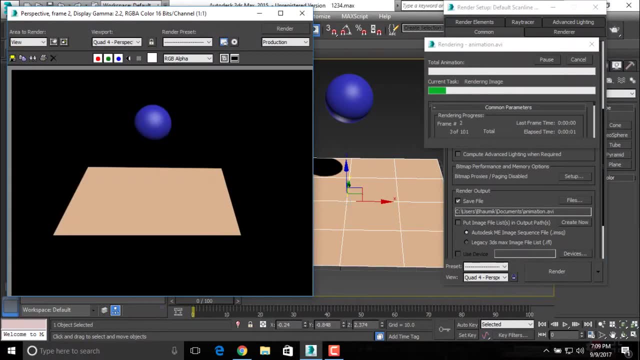 render one by one. all frame is rendered one by one. all frame is rendered one by one. all frame is rendered. now click on the render, then go to red discipler and growth. now click on the render, then go to red discipler and growth. now the render is rendered. so in my case in red disc. you can see during this Truly 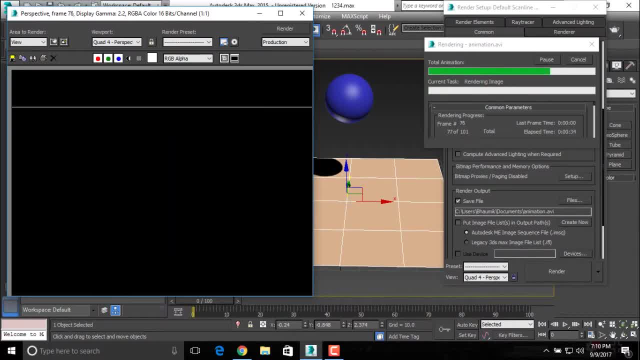 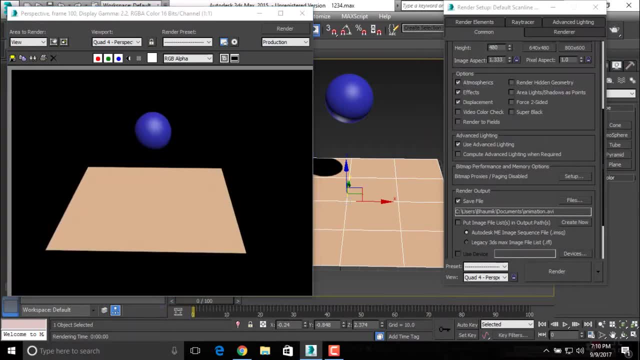 rendering display. you can go further and remove all the any key elements so that your both active file can from 0 to 100 frames, because we want suitable camera effect from 0 to 100 frame when active one time in the 56 2020 is for that we are. 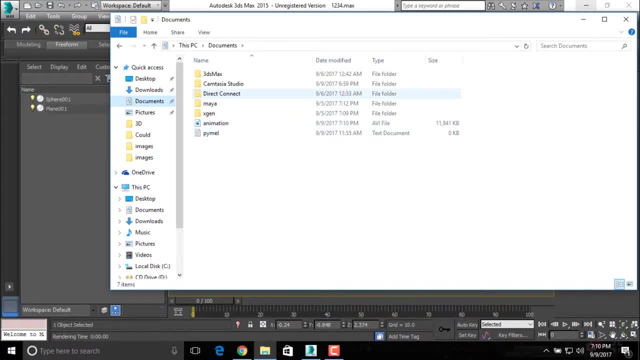 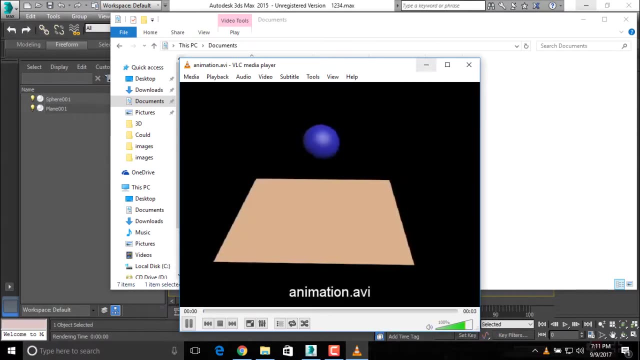 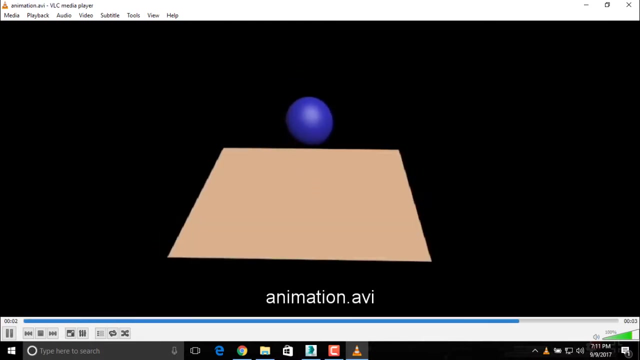 certainly running out of multi data information going around and explaining. in the on the you can see your animation. this is our animation file. I will open it with the VLC. you can use any software for open your AVI file. so our animation is done. this is a final rendering output. we are created in 3d software.